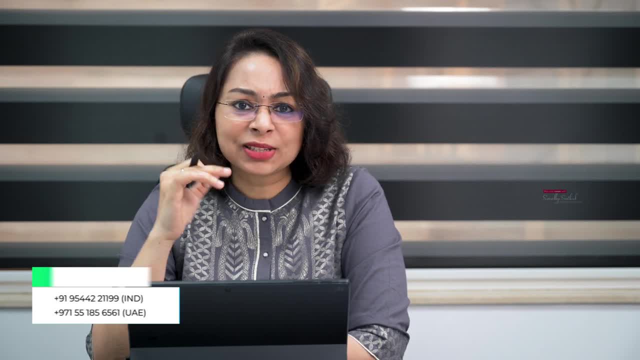 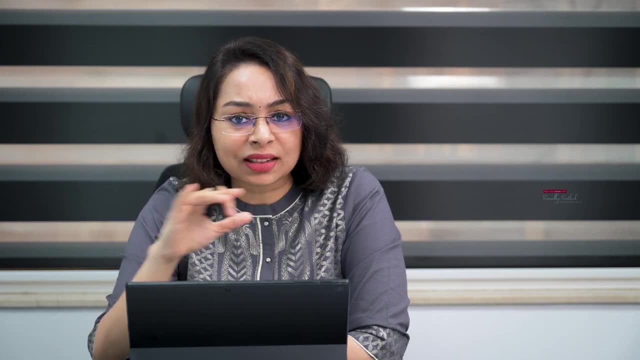 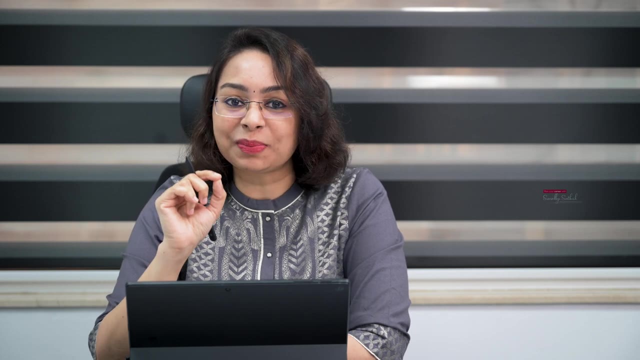 who delivers courses related to aerospace. So in the comments of that video there are a lot of people who have asked to explain the courses that they have, as well as the other courses that are related to aircraft, aerospace and things like that. So in this video I am going to 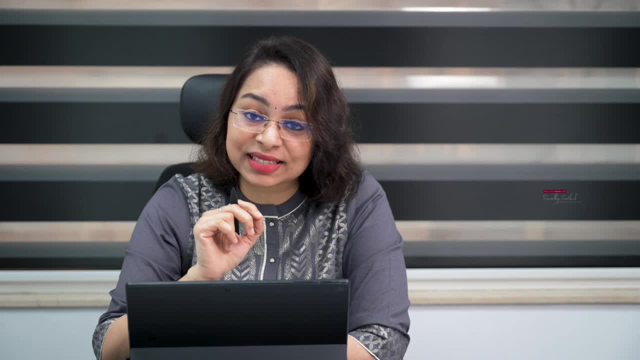 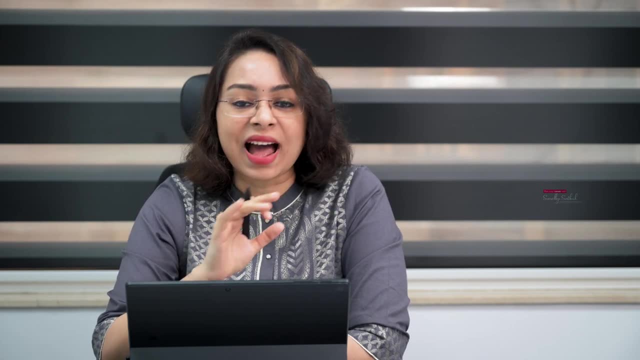 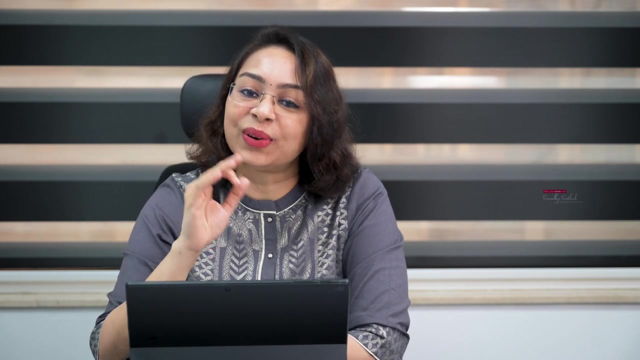 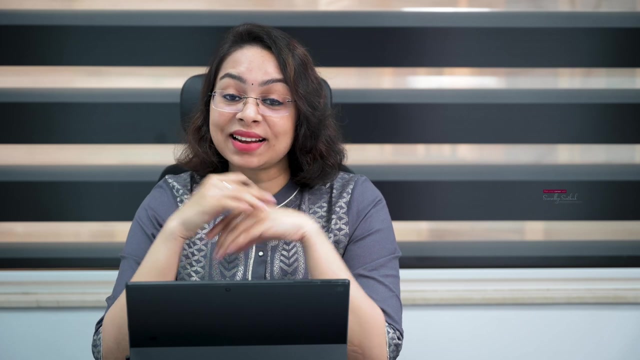 specify two different courses, which is avionics and aerospace engineering. that is offered by Indian Institute of Space Science and Technology and will explain you every detail about what you will be studying if you take up that course after your grade 12.. When it comes to things that are flying and space, you have a lot of courses that can be. 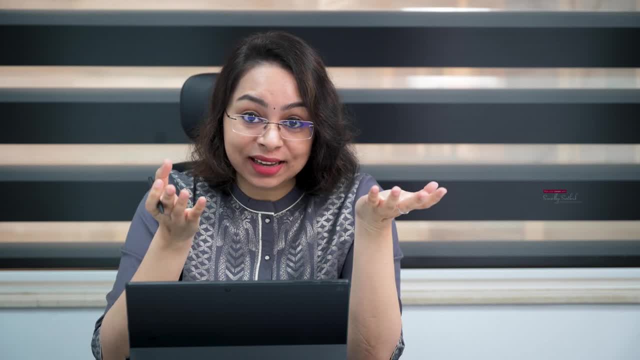 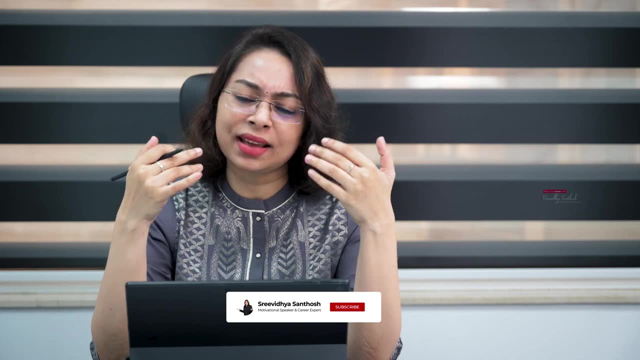 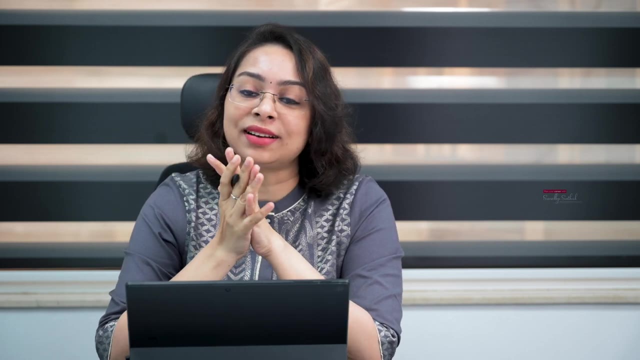 pursued after grade 12, like your aeronautical engineering, aerospace engineering, aviation physics, avionics, aircraft maintenance engineering, etc. And there are a lot of colleges and universities in India that provide these courses for the students after completing grade 12.. Even in India, there are a lot of colleges and universities in India that provide. 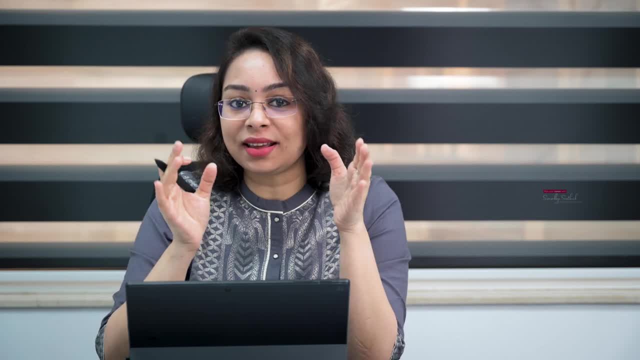 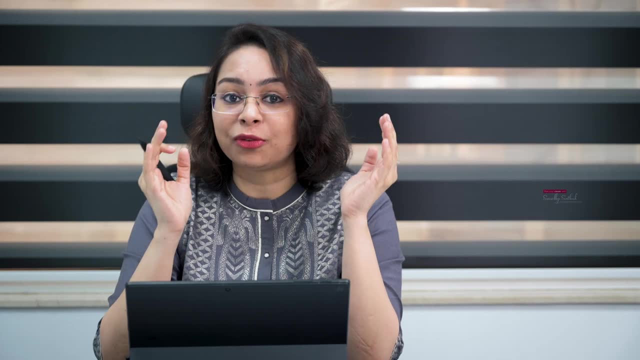 these courses for the students after completing grade 12.. Even then, I would say the best of the institute for studying these courses would be IISD. Always aim for premium institutes if you are planning to pursue any of these courses. When it comes to IISD, there are three different. 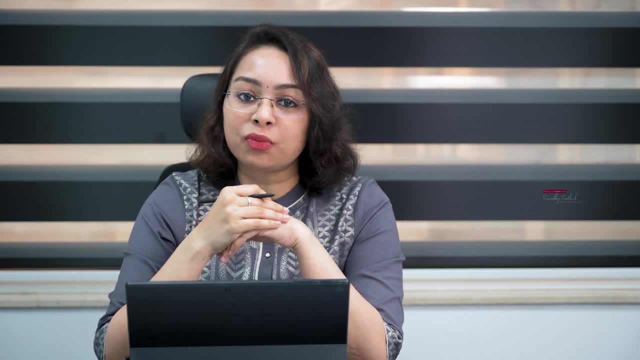 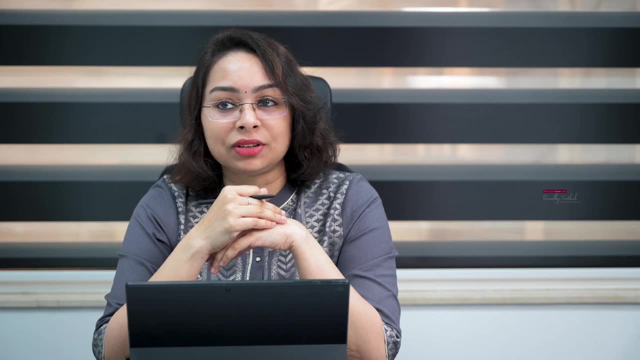 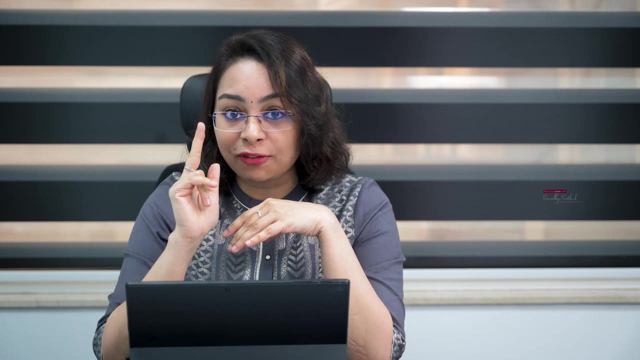 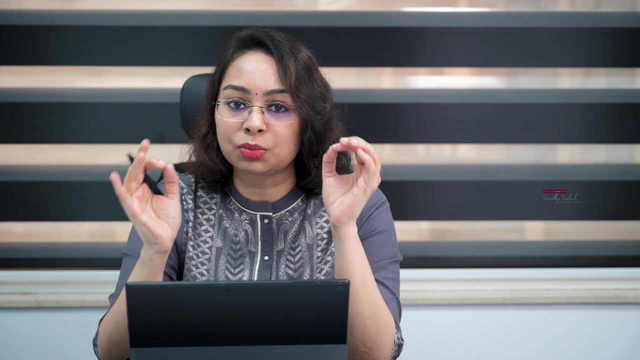 courses that you can pursue after your grade 12, of which one is BTech in aerospace engineering, another is BTech in electronics and communication engineering, specifically avionics, and the third one is a dual degree program. In this video, I'm going to specify about the first two programs of IISD. Don't think that IISD is the only institute that provides these programs for you people. 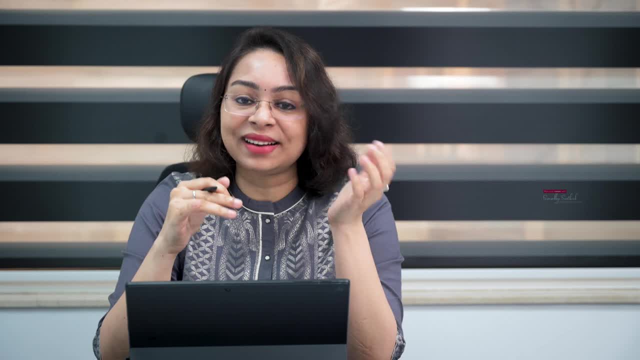 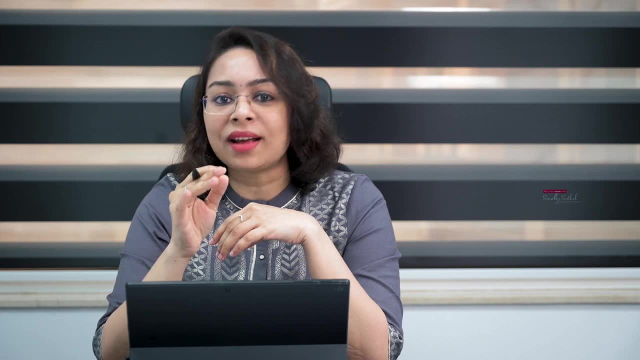 There are a lot of other universities too, but, as I said earlier, the best of it in India would definitely be IISD, And if you want an admission in IISD, please check my previous video, which is given in the i button. 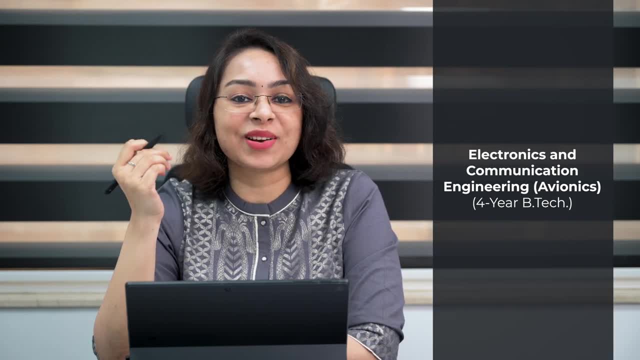 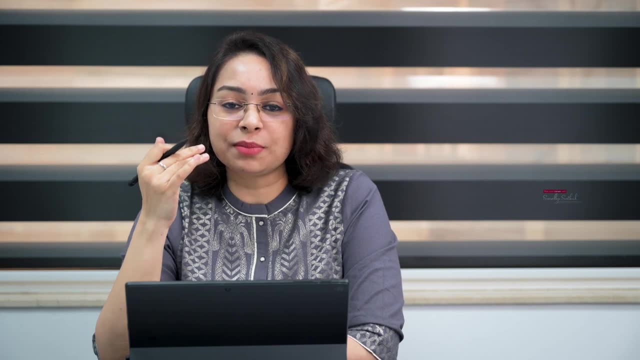 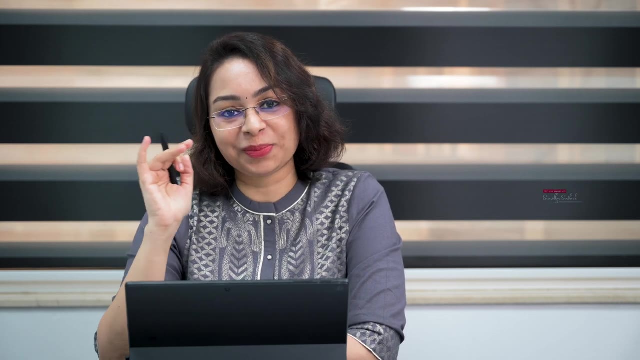 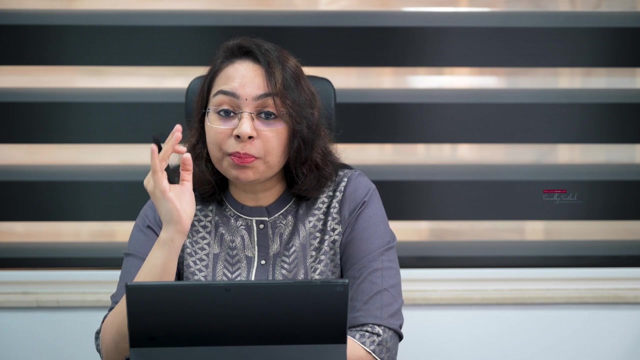 If you want to study more about the communication system that is used inside a spacecraft and aircraft, this is the course that you need to pursue. Hope, all of you know the importance of communication system in any aircraft, how important it is to communicate between this. 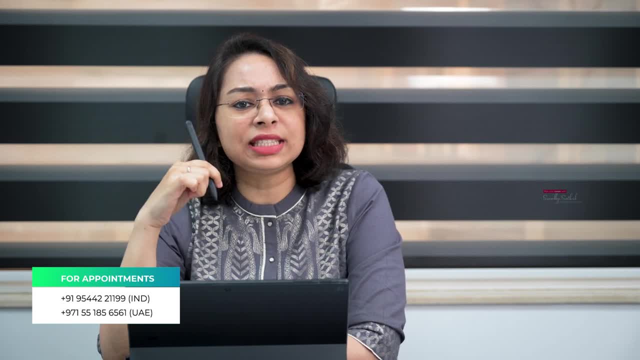 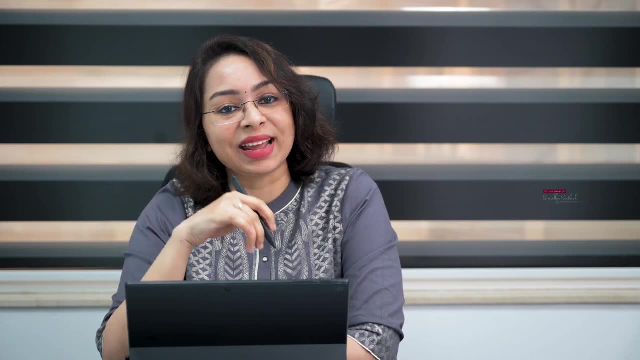 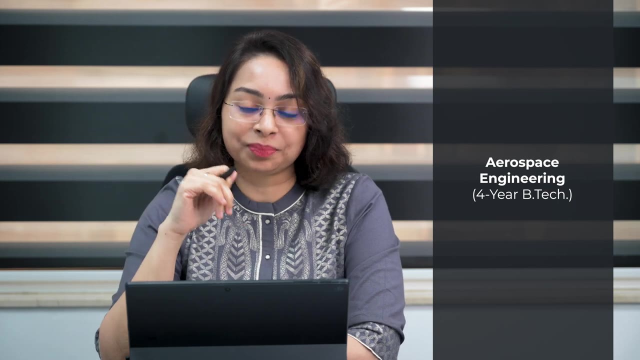 aircraft as well as the ground system. If you want to design and devise various things which are related to these things, pursue your BTech in avionics after your grade 12.. The second course that is available in IISD is called BTech in aerospace engineering. 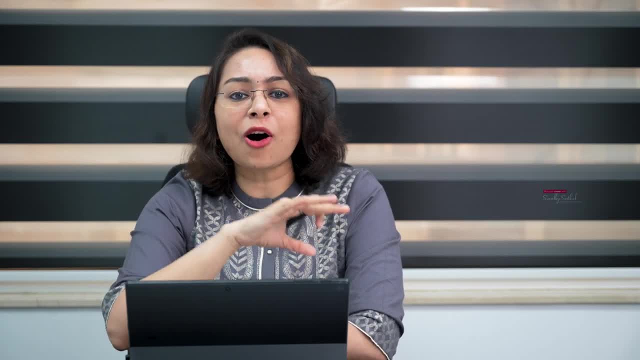 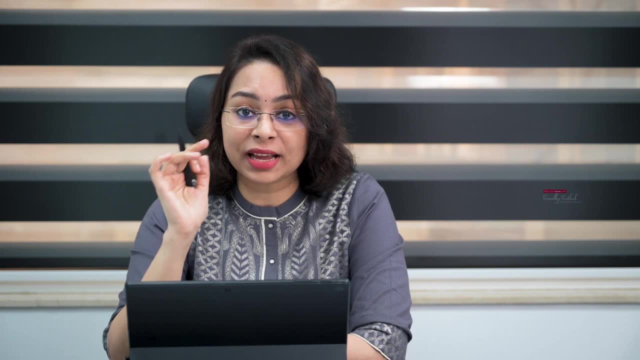 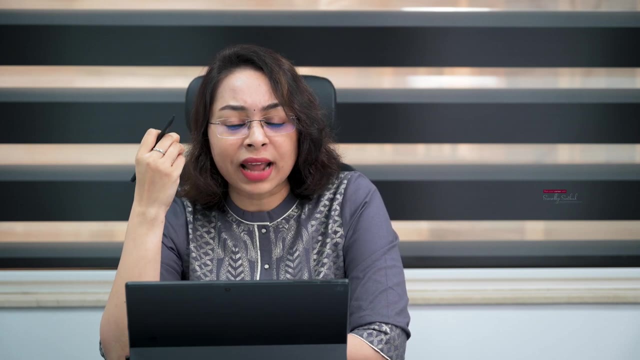 When you pursue aerospace engineering, you learn a lot of things which are related to spacecrafts and aircrafts. Now, aeronautical engineering is a little different from aerospace engineering. If you also want to know about details in aeronautical engineering, or even aircraft maintenance engineering, do drop the comments. 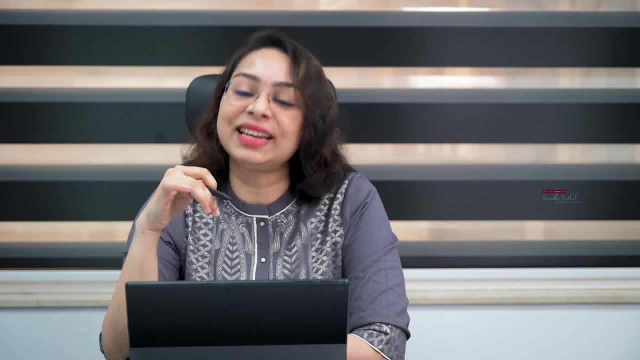 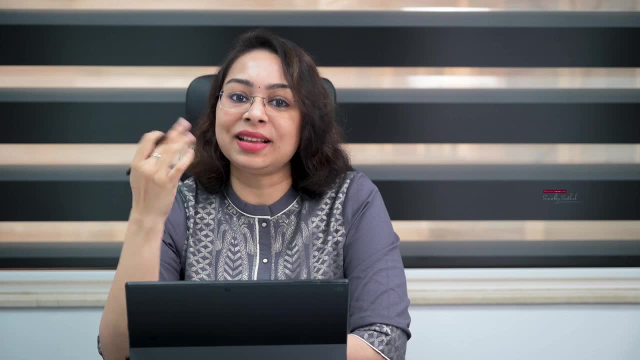 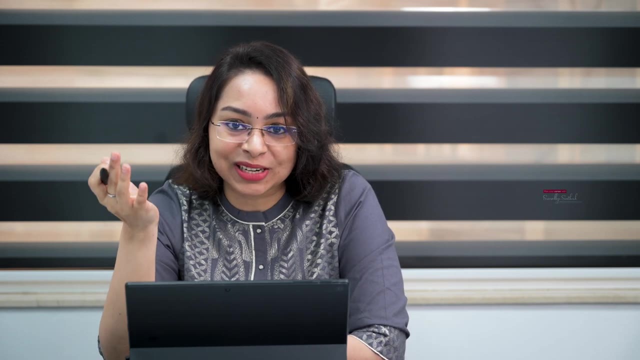 in the comment box so that I can explain about all those courses in an other video. Coming back to BTech, in aerospace engineering you can design aircrafts and spacecrafts like airplanes, helicopters or rockets and lot many things as such, And also you can plan missions. 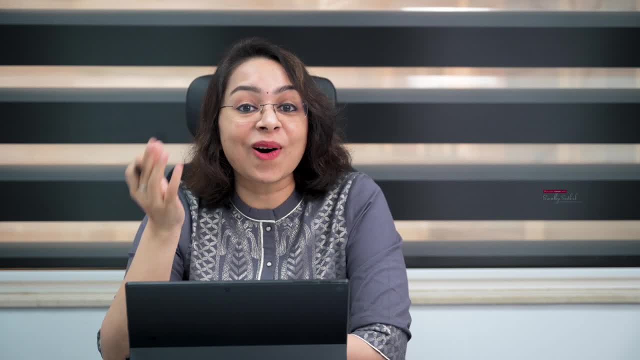 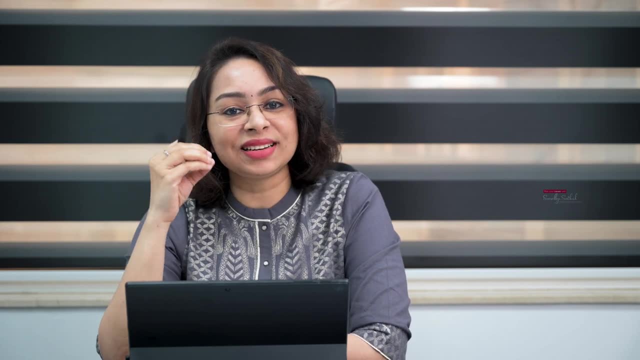 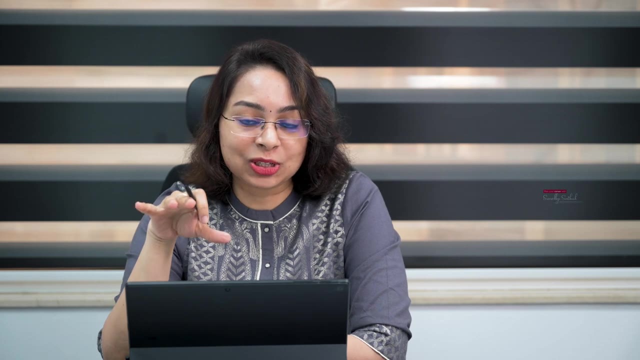 missions like Mangalyaan, Chandrayaan, and also you can plan trajectories. Doesn't it sound amazing? So those students who are really interested in getting on to things like this can pursue a BTech in aerospace engineering. Also, let me remind you, IISD is not the only place for these courses. 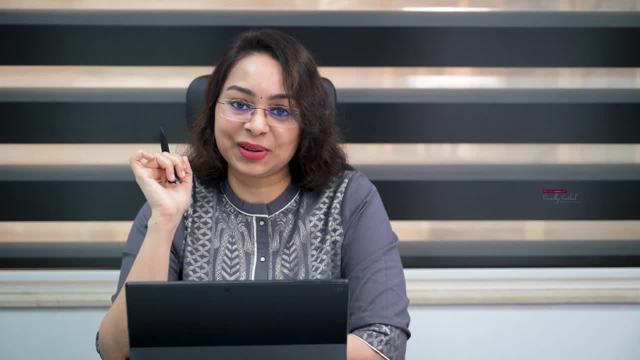 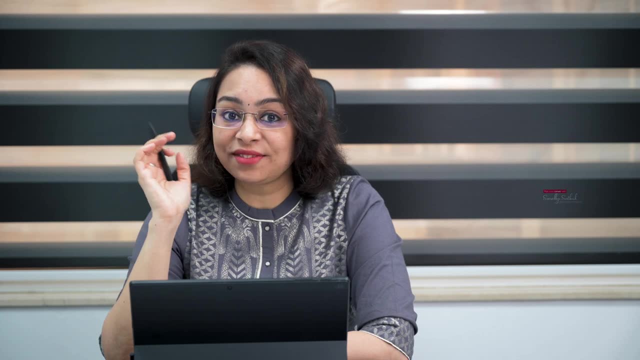 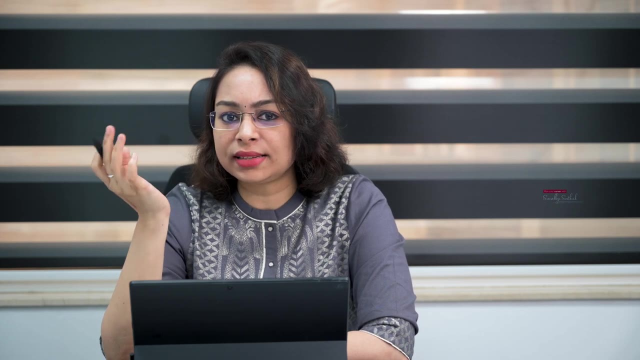 You have lot many other places, but these are the premium institutes, As you all know. you should have taken Physics, Chemistry and Mathematics and mathematics for your grade 11 and 12 for pursuing any of these courses. there are some children who says like this: okay, i hate chemistry, but i love mathematics and physics. still, i want. 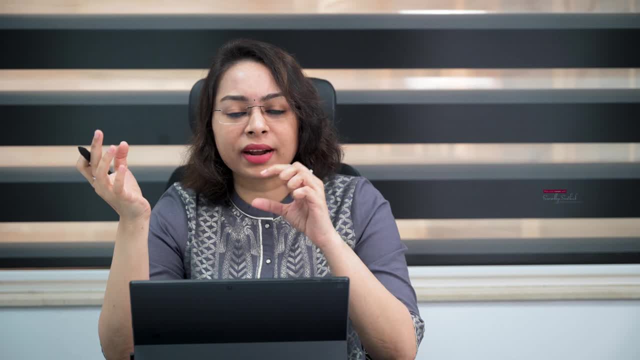 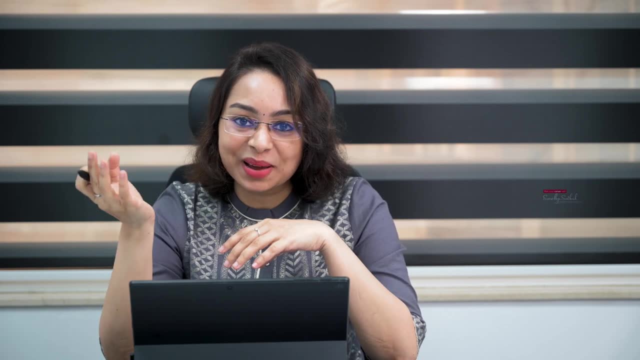 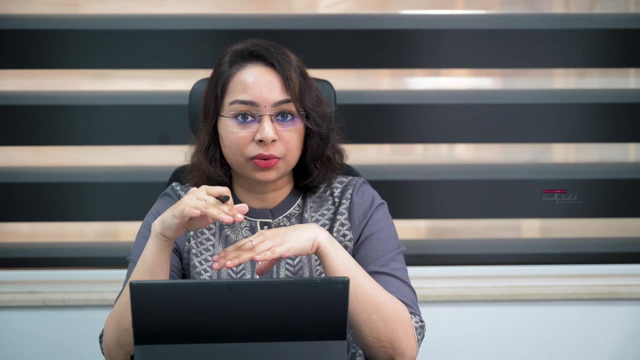 to pursue engineering. okay, because there are a lot of engineering programs where chemistry plays only a very small role. but when it comes to courses like aerospace engineering, don't say like this, because you will not be able to learn fuels or fueling systems without chemistry, so chemistry will also play a crucial role in this program. so don't hate chemistry and get on to. 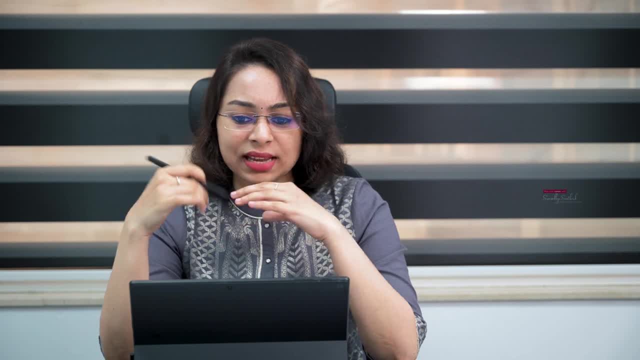 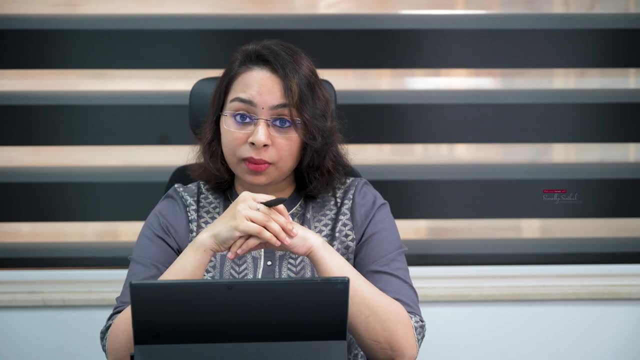 these programs, there will be a few children who always says like this: i don't want to study for a long number of years after my grade 12. i'll just finish my graduation and then try to get on for a job. so if you are having this sort of a mindset, i'll ask you to think twice before getting into. 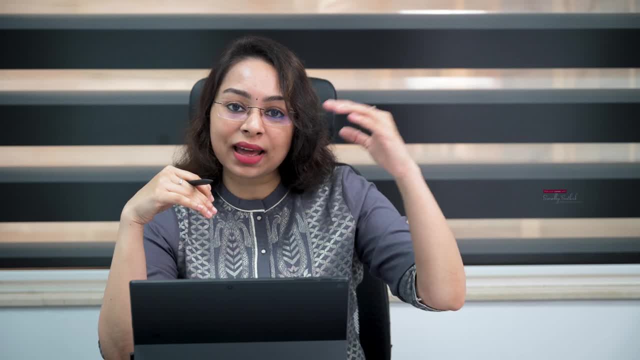 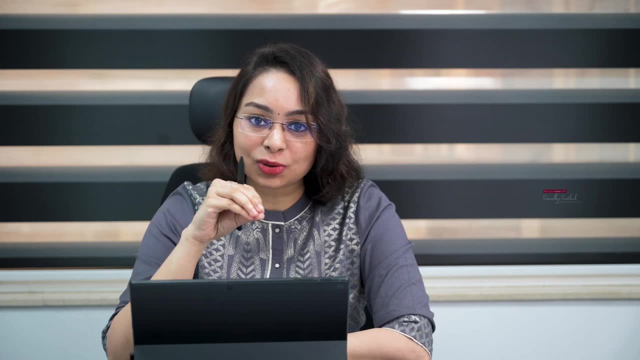 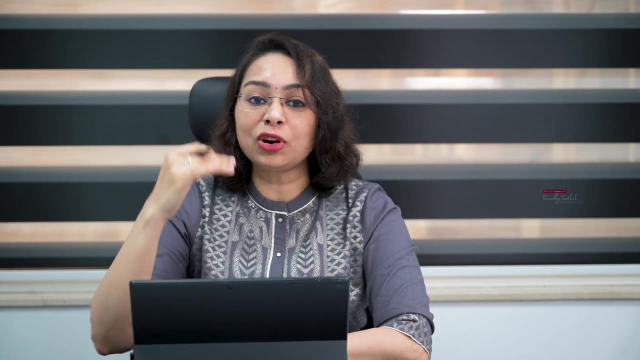 any of these programs. because if you want to get into a higher level of your career, you should complete your bachelor's, master's and even do your phd, because a lot of children who get into these programs will always be dreaming of places like isro, nasa, drdo, etc. so if you want to get into those levels and climb up the career ladder, 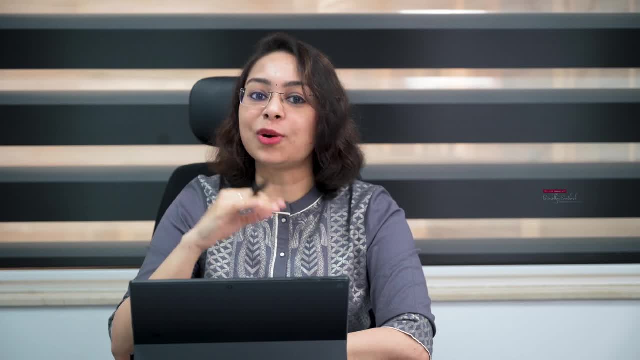 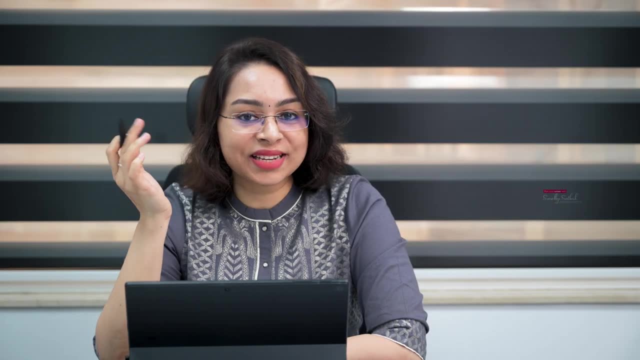 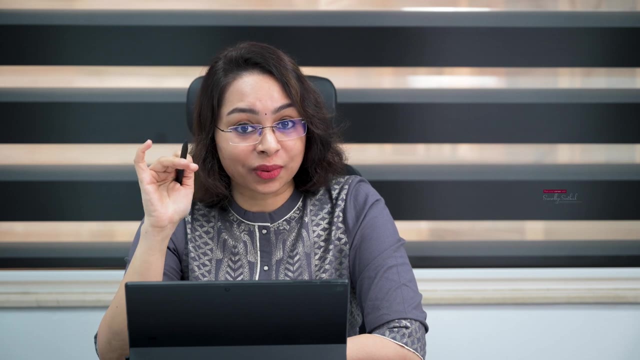 you should complete your graduation master's as well as your phd program. creativity, innovation and analytical ability would be the main three traits that you would require if you want to pursue any of these programs. you should complete your bachelor's, master's and even do your phd. 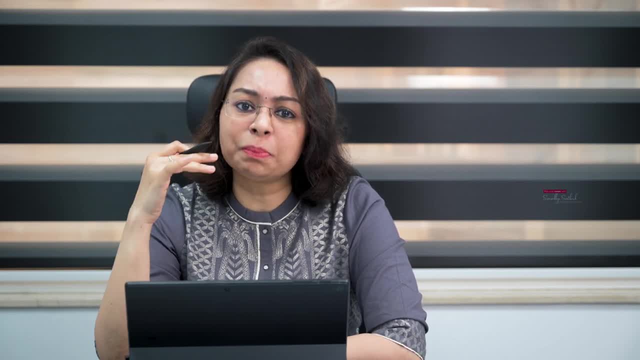 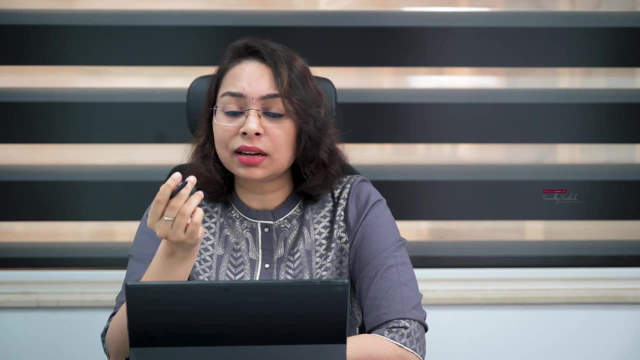 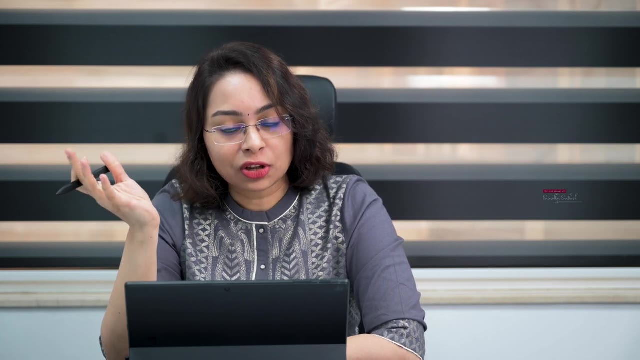 think it from a practical point of view: whenever there is a mission, there are a lot of things that you have to take care, for example, fuel consumption. even a small milliliter of fuel, if you could save it, it makes a lot of difference. so if you want to understand and design and devise things, 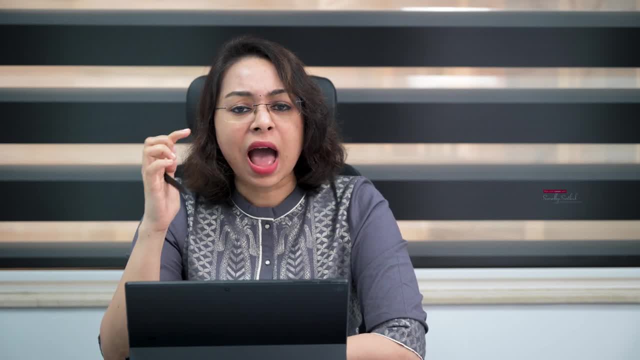 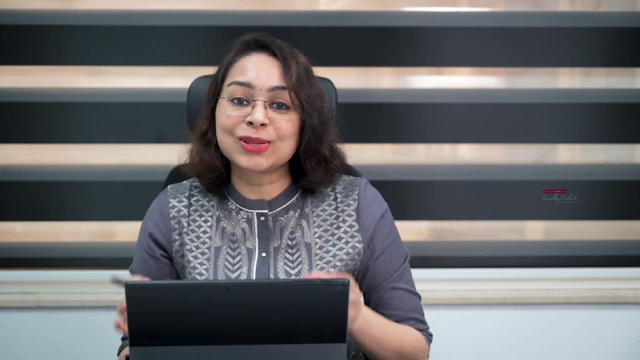 accordingly, you should have an analytical mindset and you should be able to innovate and find out new, new things that can be done in your life. so if you want to get into a higher level of your profession, so you should have a background like engineering code, but if you need more. 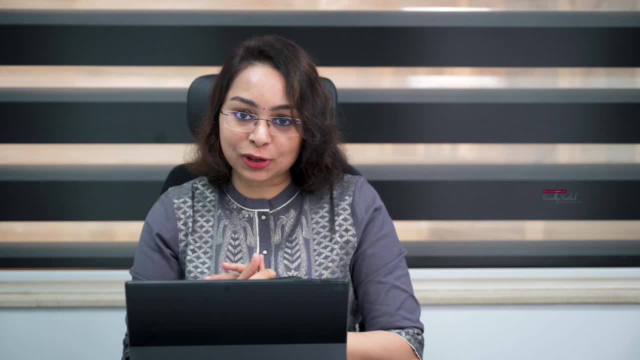 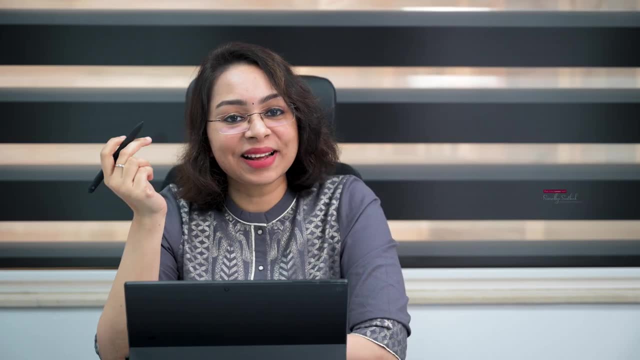 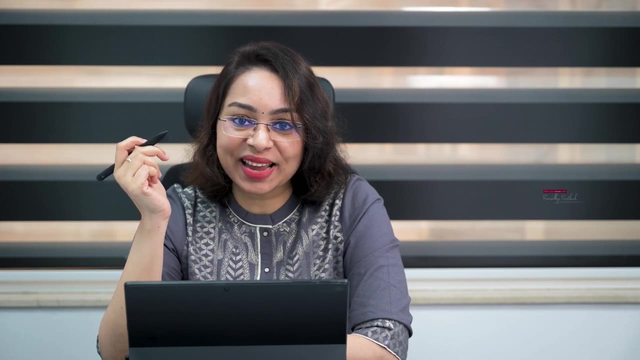 knowledge, or 차�, as well. you should work hard towards the in line levels, right? so training chemicals. I'd be mindful about what I'm going to study, exactly what will make me successful, and I'm not so sure I don't have enough knowledge in this market. what I haven't found out is: 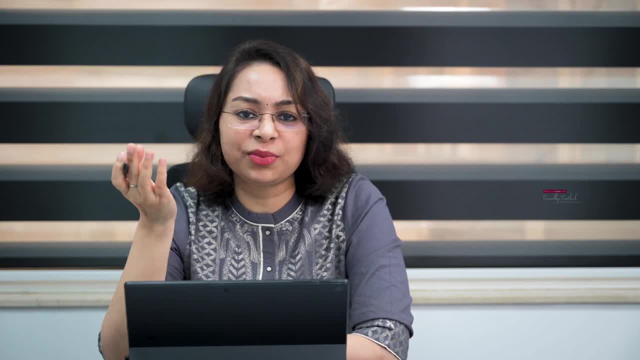 that this profession offers new things. change your £$ польз a year, just. the project gets better, faster. and now you wanna start something else, right? so you want to take care of production benefits? do you want to work in related jobs? do you want to exercise assignment every dayin your courses? these are goals. those are gradient steps that are important to help with your career mission. where is that? a great 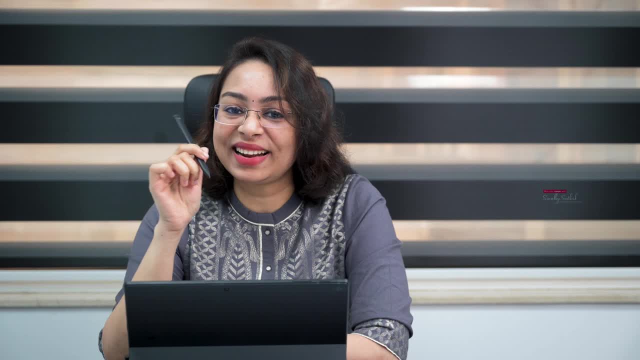 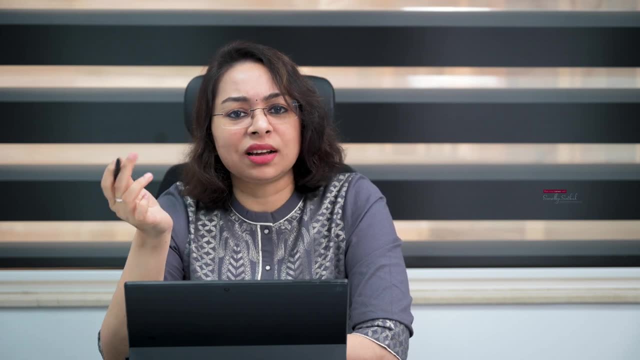 you should also be thinking of the private institutes, but there are a lot of things that you have to keep in mind if you are planning to get into a private institute. like these, courses are not just theoretical studies. it has got a lot of practicals to it, so the institute should 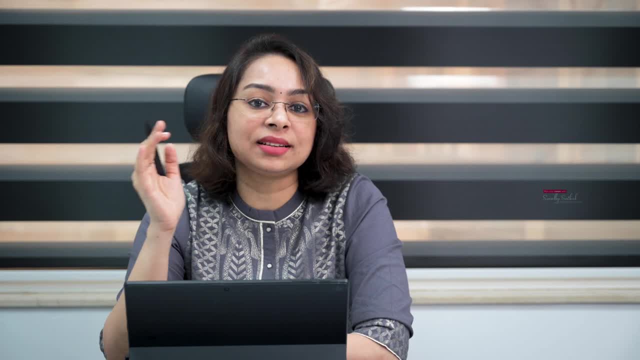 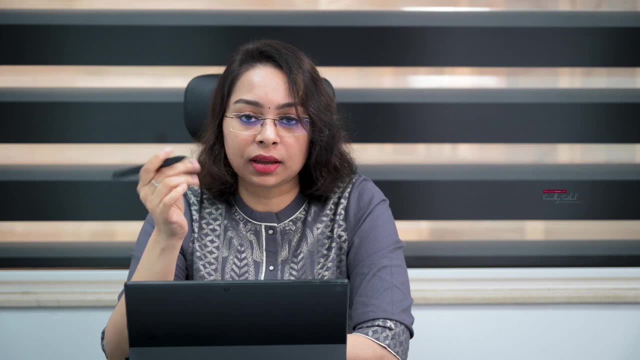 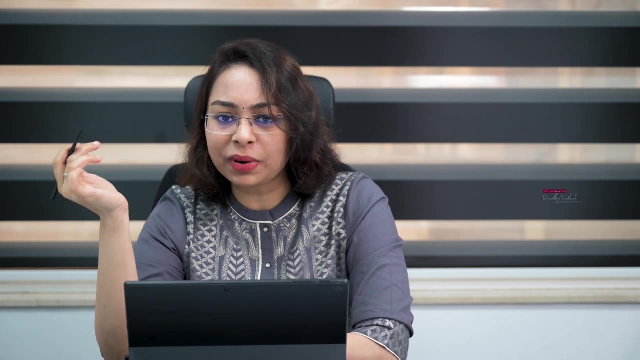 have enough of facilities to give you the practical learning. the faculties should be skilled enough to impart their knowledge. third, and most important thing, in most of the places you will have an internship towards the end of the semester. so when you go for an internship, if you are from a premium institute, it will be far easier to get an internship compared to a student.